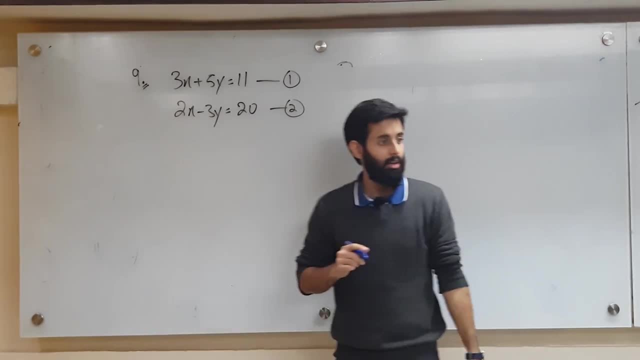 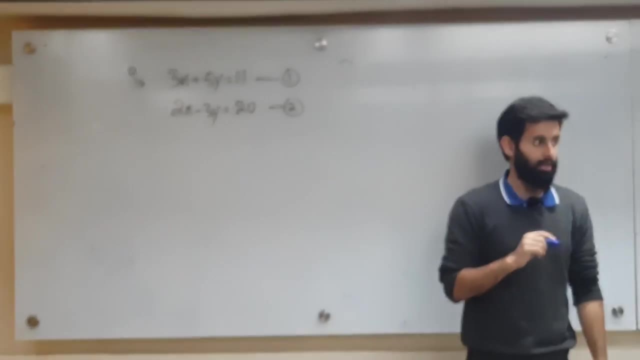 What have I decided? I'm going to solve this question by substitution. Now listen to me In this: if I decide to go with substitution, then what will I have to do? What will I have to do? I'll have to make a subject out of any one equation out of any one variable. 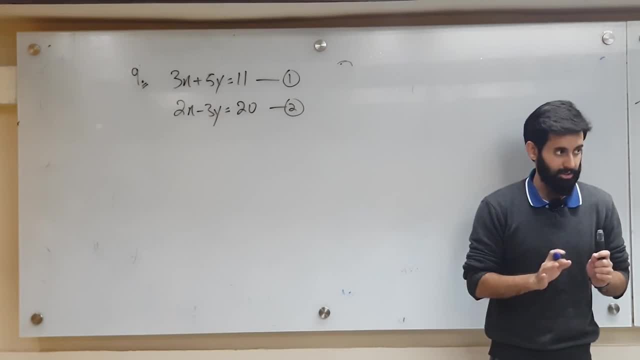 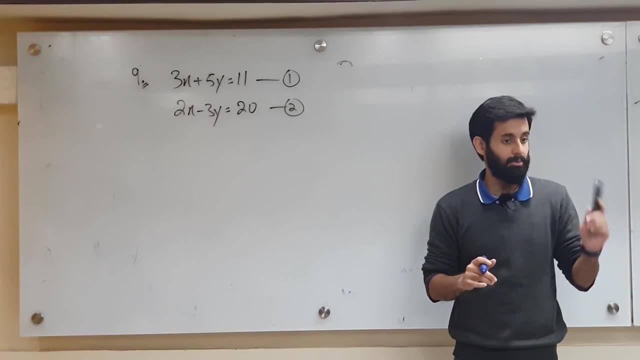 What have I said? I'll have to make a subject out of any one equation, out of any one variable. Manu, repeat, Manu. what did I say? Out of any one equation, out of any one variable, I'll have to make a subject. 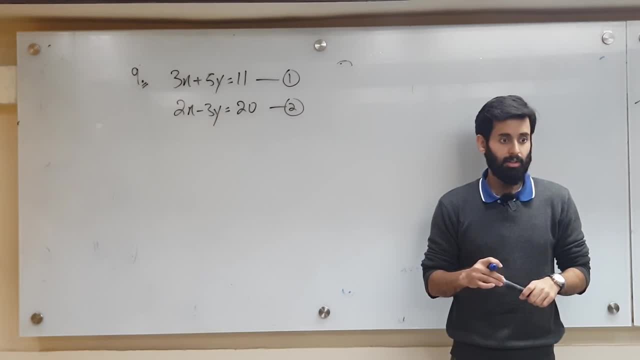 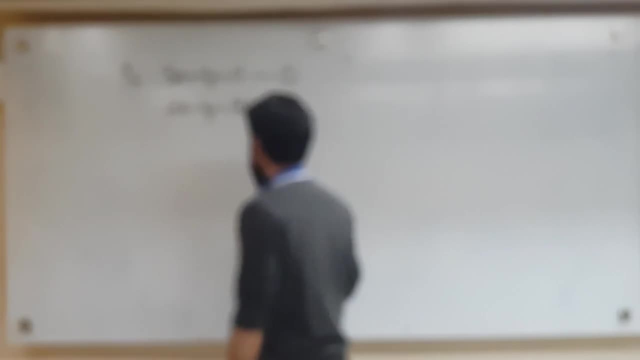 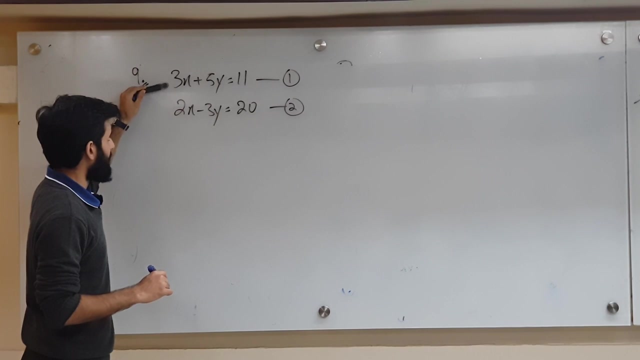 Yes, it's not necessarily at all. I've decided to solve this by Substitution. Okay, now suppose I decide to take equation number 2 and make x the subject. Okay, remember, as I always say, take simpler of the two equations. 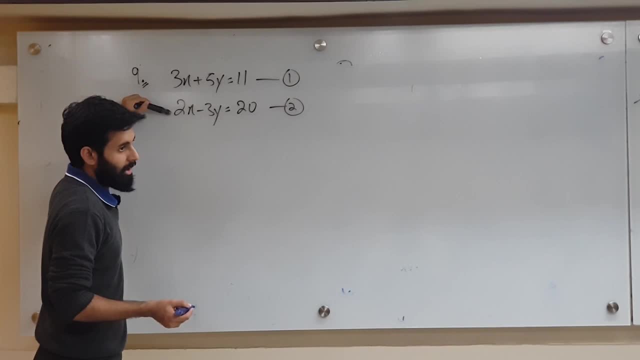 Now here. we don't have any simpler equation. Why? Because in every equation there's either a coefficient of x or a coefficient of y which is other than 1.. Okay, So if I make x the subject out of equation number 2, so what do I end up with? 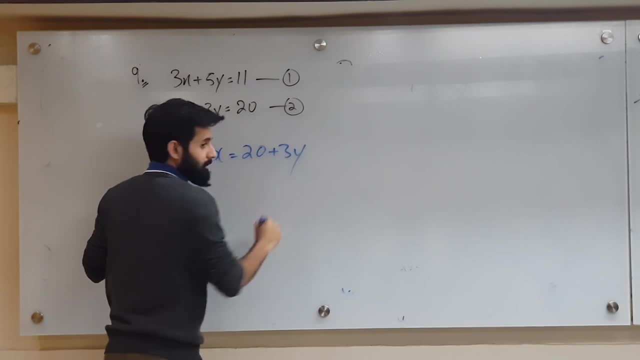 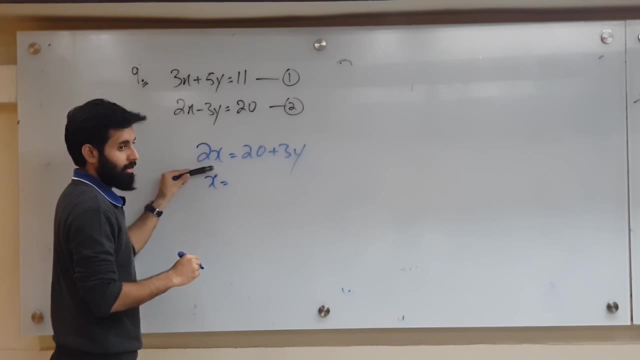 2x equals to 20 plus 3y. Did you understand what I did? You said 20.. Now if I, What's 2 and x doing here? Alina, What's 2 and x doing here? What's going to happen if I go there? 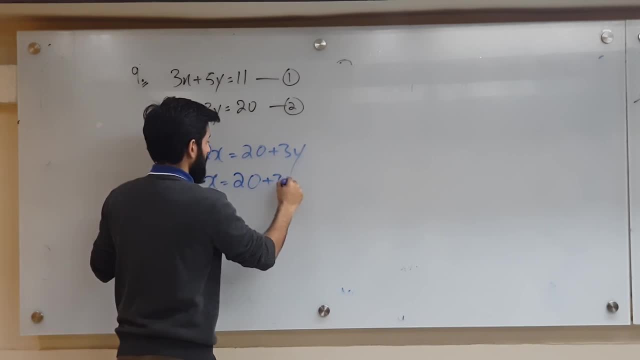 What's going to happen if I go there? It'll divide, It'll be 10.. So 20.. No, no, no. 20 plus 3y upon 2.. That's it Now, don't do this. that 2 ones are 2 tens. 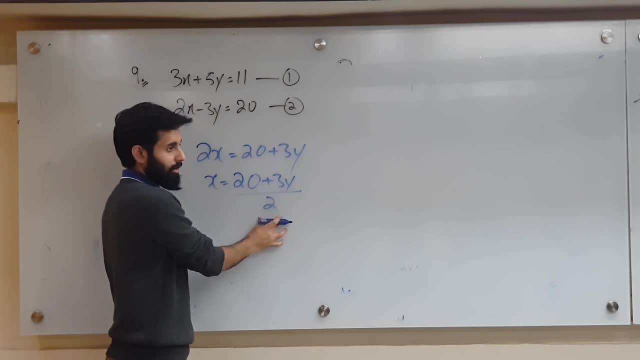 No, no, no, no. Okay. Why? Because this whole thing is divided by 2.. It's not just 22 that's being divided, 20 plus 3y upon 2.. Okay, So what have I got? 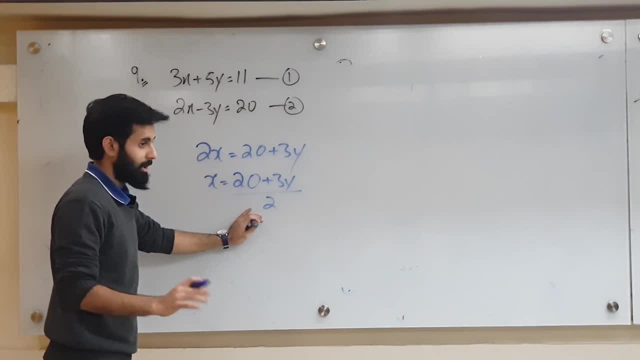 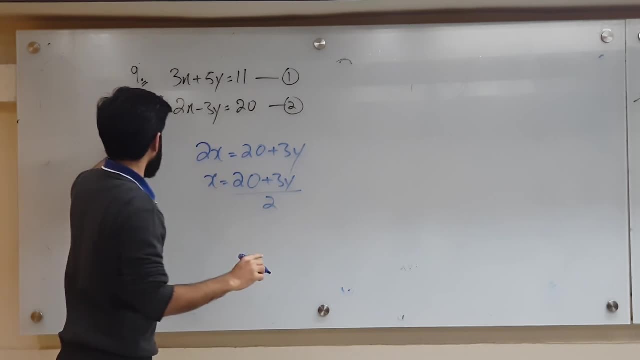 I've got x subject. What's it become? x subject, x subject: With whose help has this come? With which equation's help has this come? I'll plug it in equation number 1.. In whose place will I do it? 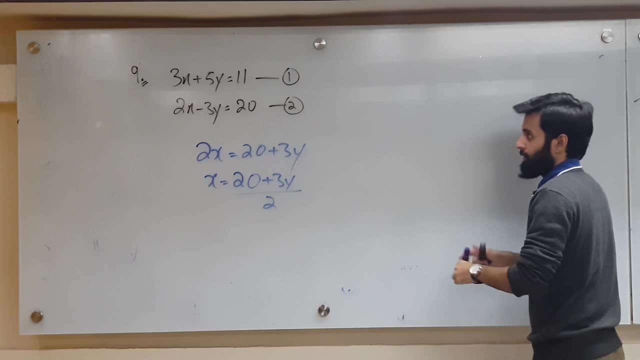 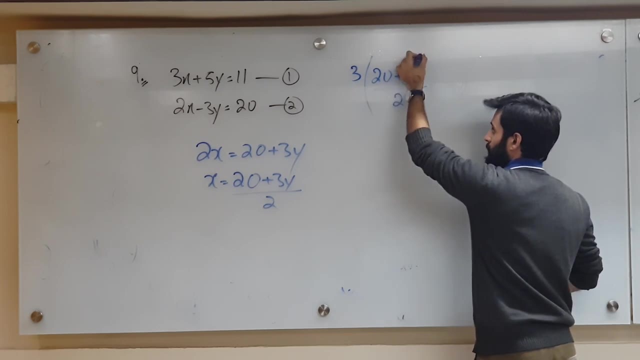 In x's place. Okay, Let's solve this here. So here we have 3.. What will come in x's place? 20 plus 3y upon 2.. That's it. Any questions so far? Plus 5y equals to 11.. 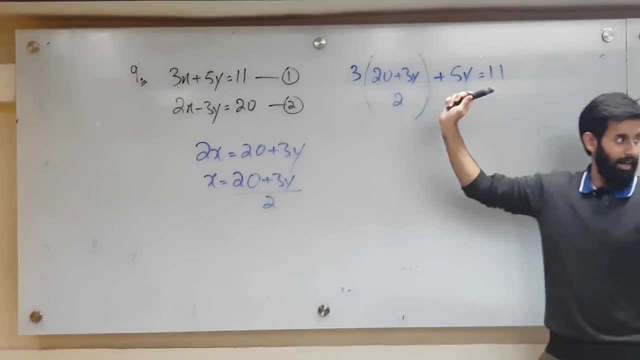 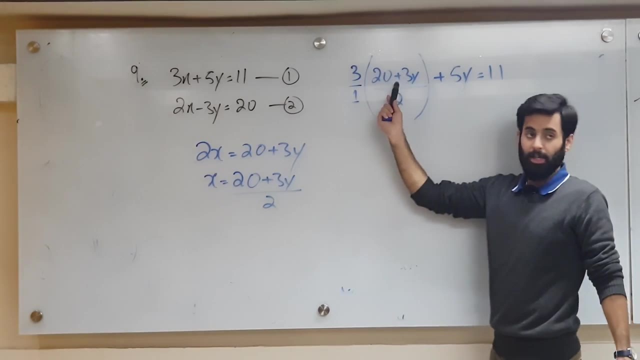 Very good. Now how will this 3 be multiplied? It'll be multiplied by the numerator. So what's? Because? 3 means what It's: 3 upon 1, right, So 3 will be multiplied by the numerator of this fraction. 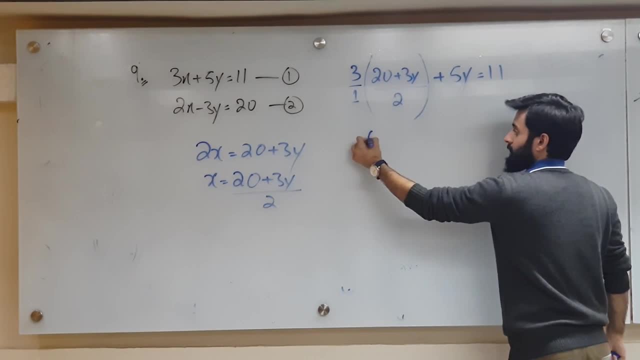 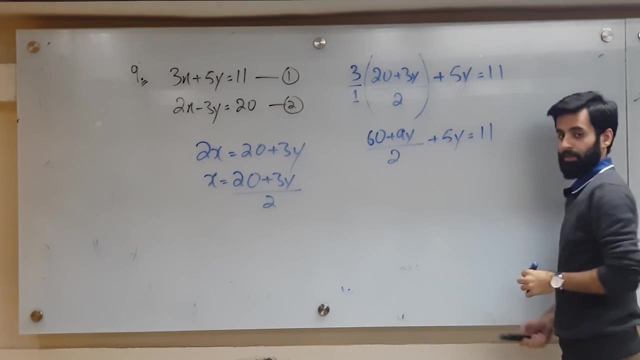 and 1 will be multiplied by the denominator of this fraction, 60 plus 9y upon 2.. Very good, Plus 5y equals to 11.. What can we do now? How about I take out the LCM? What will be the LCM of 2 and 1?? 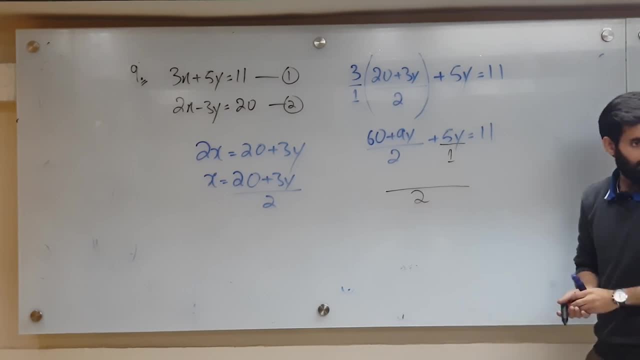 2 will be there, right? So yeah, Now what will we do? This will stay as it is 60 plus 9y As it is Plus 10.. Plus, To make it equal to 2, I'll multiply it by 2.. 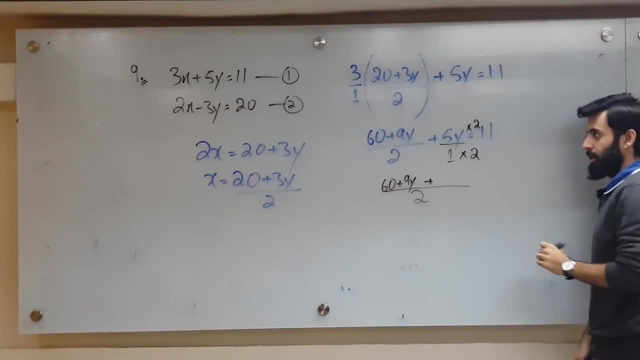 So I'll multiply the numerator by 2 as well 10.. So what will it become? Let's do this: 2 into 1.. Right, 60 plus 9y into 1.. Will stay 60 plus 9y. 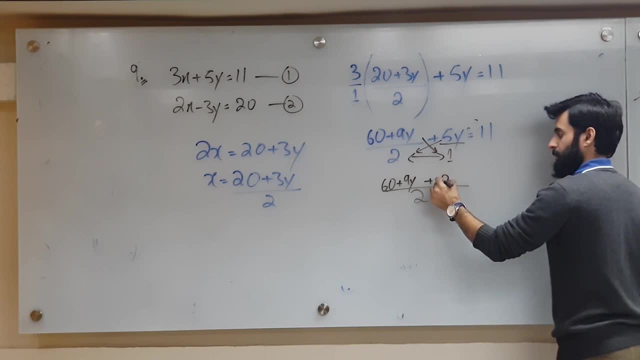 And 5y into 2, what will it become? 22 minus 60. Right Plus 20.. Sorry, Sorry My bad- Plus 10y Equals to what? Equals to 11.. Any questions so far? 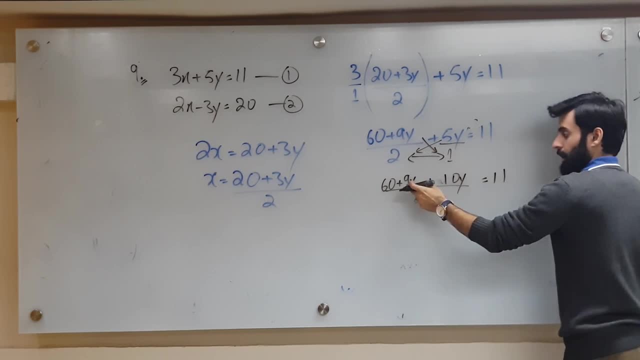 1 over. We'll put 1 over 11.. We'll put 1 over 11.. No, no, no, Yes, Okay, let's put 11 over 11.. Let's see if we can add or subtract anything here. first, 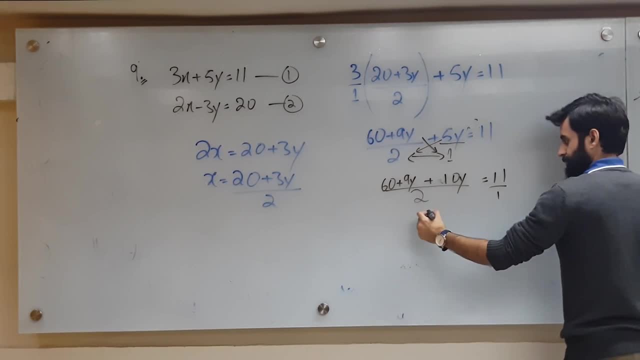 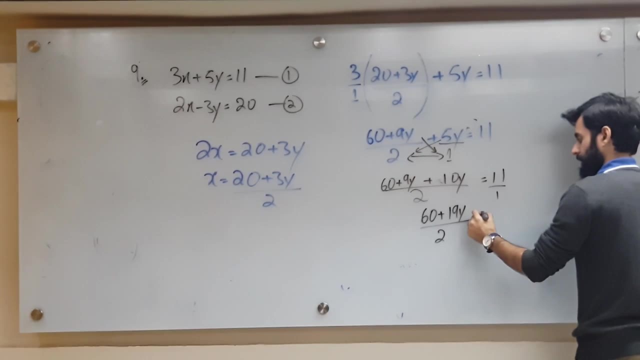 Yes, yes, Do you have like terms? You have 9y and 10y, 19y. So 60 will remain as it is, Plus 19y. Let's not use a calculator. Let's not use a calculator. 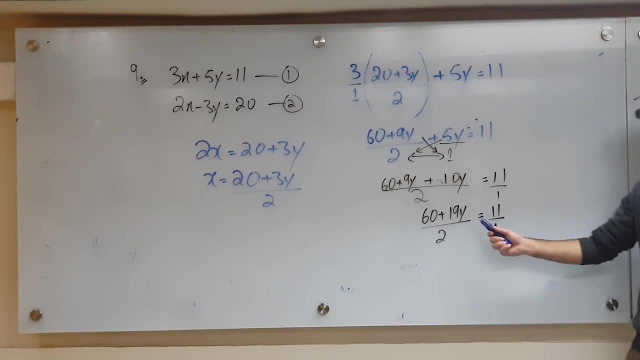 Equals to 11 over 1.. Umar, let's not use a calculator. Still, let's not use a calculator. What's 60 plus 19y into 1? Same here, Umar, Who will get the penalty? 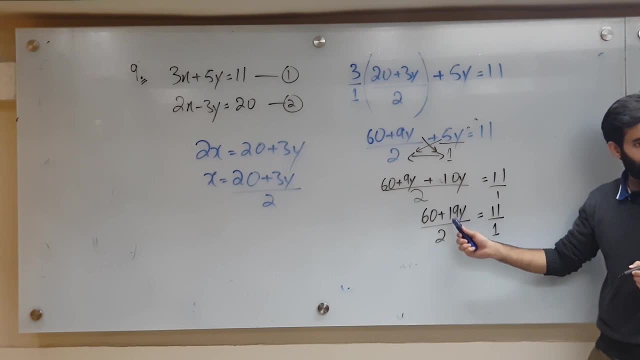 Hey, cross multiply. Yes, sir, 1 will go there, 2 will go there 2.. Uh, When 1 will be multiplied by 60 plus 19y, will it make It won't be cross. No, no, no. 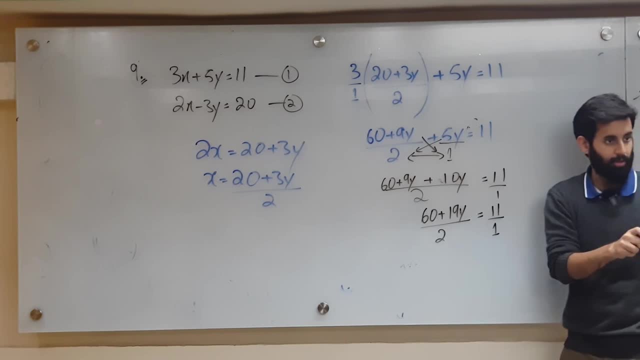 There's an equals sign in between. Cross Whenever you have an equals to sign in between. whenever you have an equals to sign in between, what do we do We cross? multiply What did I say? Whenever we have an equals to sign in between, what do we do? 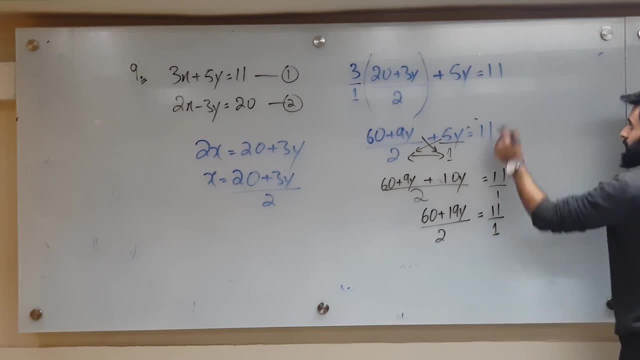 We cross multiply, We cross multiply Right. So 60 plus 19y will stay 16 plus 19y, is it Equals to 8. Equals to 22. And, as I said, let's not use a calculator. 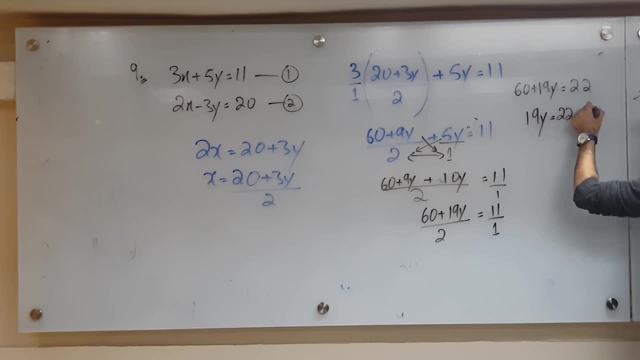 19y equals to 22 minus 60.. Minus 38.. Minus 38. And 22 minus 60 is minus 38.. Y is equal to minus 38 over 19, which is equal to what Minus 5.. 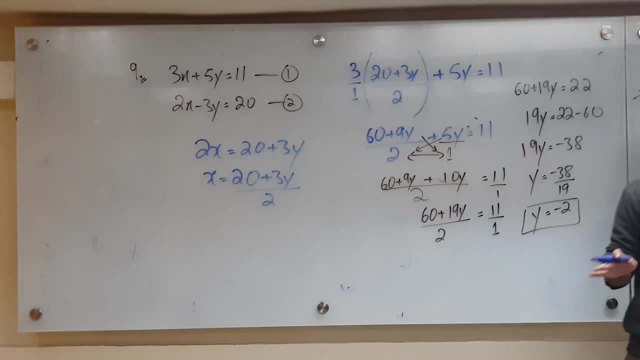 Which is equal to minus 2.. Okay, are we done? No, No, You have to put the y value into the x. Let's use this value, Find x And plug it in here in place of y to figure out the value of x. 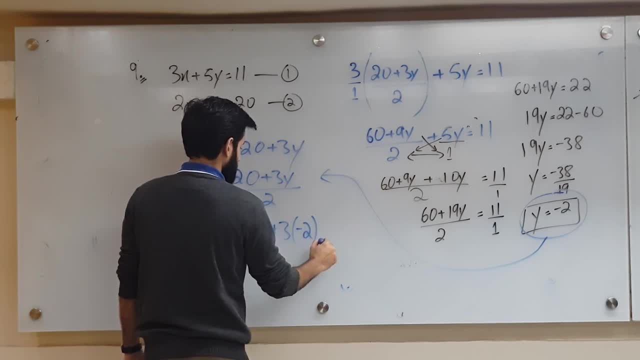 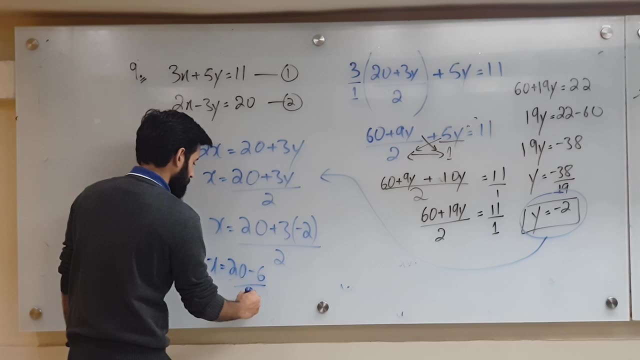 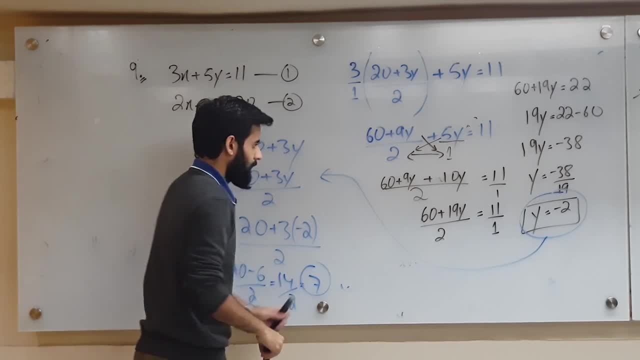 What's 14 upon 2? 7.. There you go. x is 7.. No, no, 20 minus 6 is 14.. 14 upon 2 is 7.. 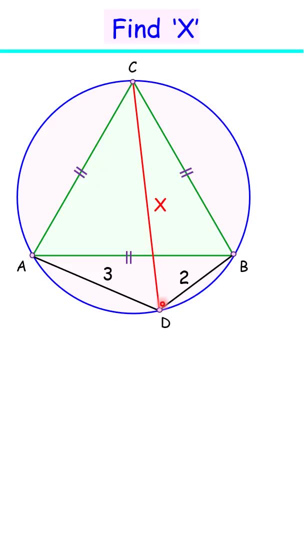 Can you find the length of chord CD where it's given that ABC is an equilateral triangle? D is a random point, such that AD and DB is 3 and 2 centimeter each. Let's start by assuming the length side length of equilateral triangle is a centimeter each. Now here ADBC. it's a cyclic. 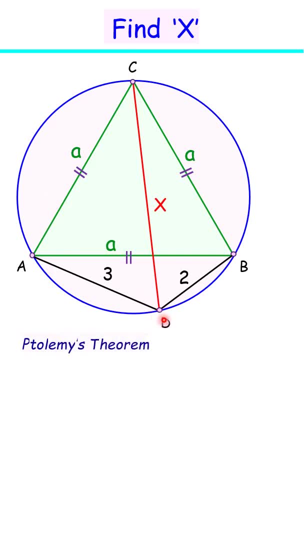 quadrilateral, applying Ptolemy's theorem in it. So it states that the sum of product of opposite sides, that is AC times DB plus AD times CB, is equals to product of the diagonal, that is AB times CD. Putting the values here, we'll get this equation. Solving it, we'll see that A is getting.